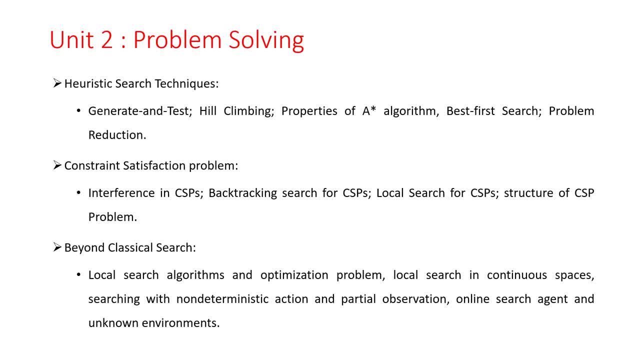 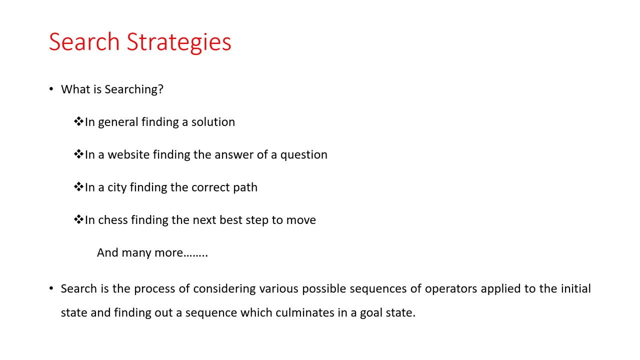 Okay, so there is a heuristic search technique, then constraint satisfaction problem and beyond, classical search technique. Okay, so in this video we are going to discuss about the heuristic search technique. Okay, so before starting about the heuristic search, First we discuss about the search strategies. Okay, what are the search strategies? So what it means searching. So searching is, in general, finding a solution. 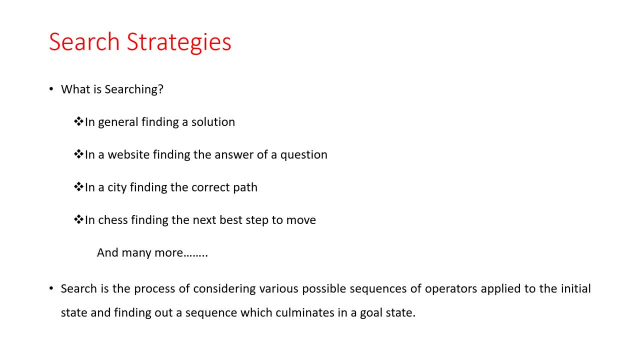 Searching is, in general, finding the website, find out the answers from the website or find out the questions. If you are having some questions, to find out the answers for that particular question oned regularly with or from the website. That means the website finding the answer for a question, city finding the correct path. 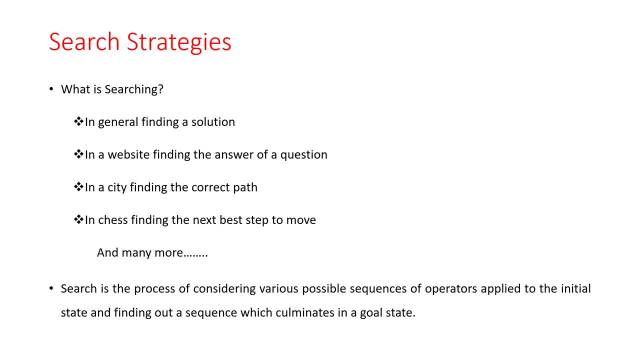 So in the city data different part from source to destination. So we have to choose the correct path To get the destination and, in the case, finding the next step to the move. So these are the different searching part. Okay, So search is the process of considering the various possible. 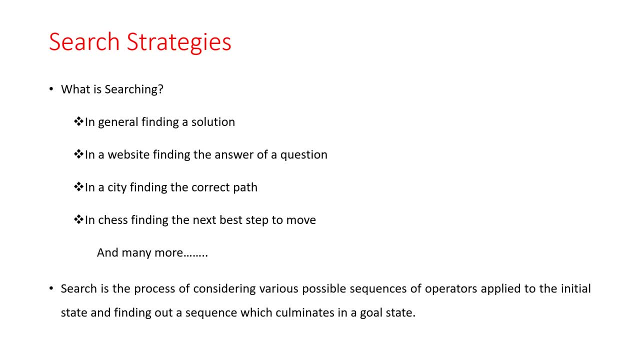 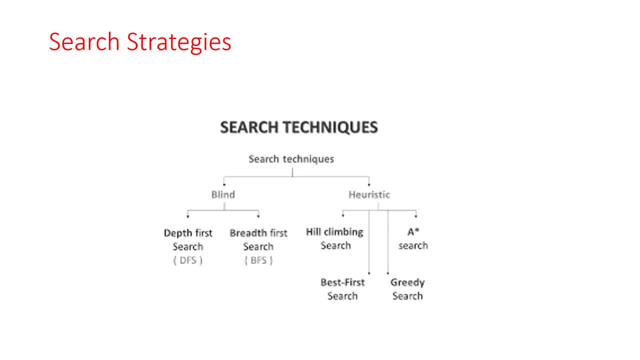 sequences of operators applied by the platform to the initial state and finding out a sequence which cumulates in a goal state. So these are the search strategies. So there is an uninformed search and informed search. So uninformed search, which is also called as a blind search, and the informed search. 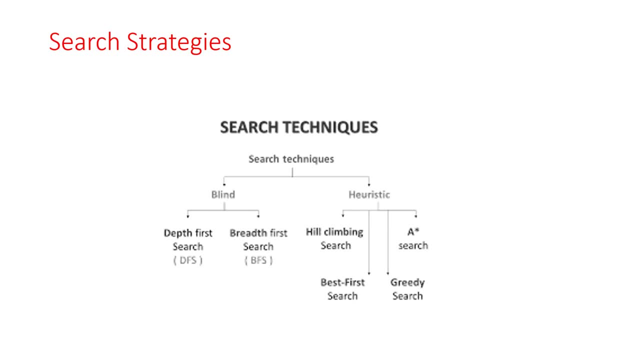 which is called as a heuristic search. Again, these uninformed search techniques are divided into the two parts, that is, depth first search and breadth first search. and in the heuristic search we are dividing this part in the hill climbing, BFS, greedy search and the A-star search. okay, 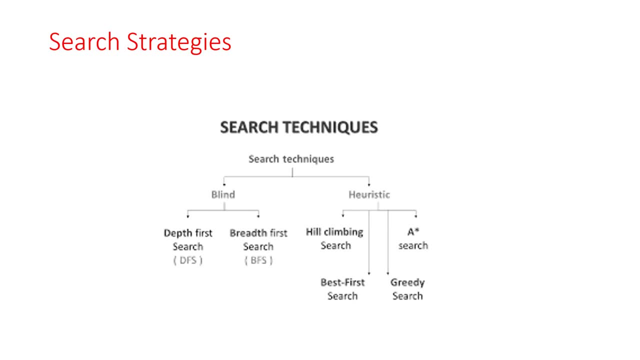 So in unit 1, we already covered the topic related to the blind search and uninformed search and we discussed this point- DFS BFS- with example in a unit 1,. okay, So I will provide the link for this: DFS BFS. 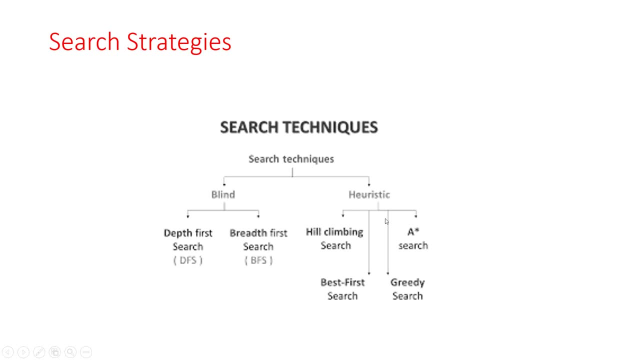 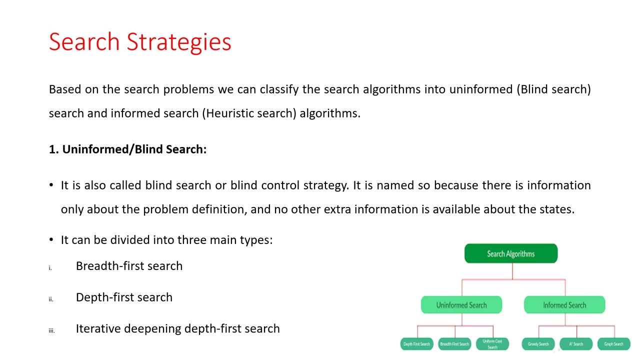 So you can check the link from the description box. So So in unit 2, we are discussing about the heuristic part, where we discuss about the hill climbing, BFS, best first search and the greedy search also. okay, So see here, based on the search problem, we can classify the search algorithms into: 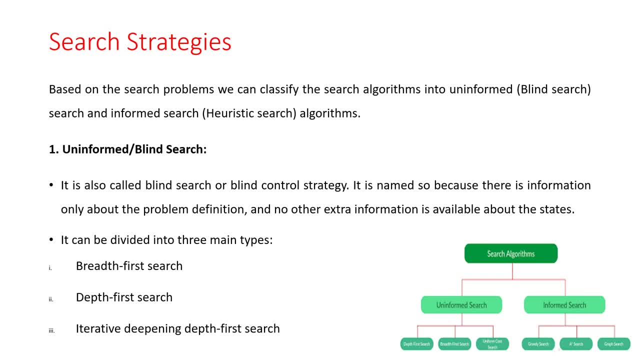 the uninformed, which is called as the blind search, and informed search, that is the heuristic search algorithm. okay, So in the uninformed or blind search it is called as a blind search or the blind control strategy. It is named so because there is a 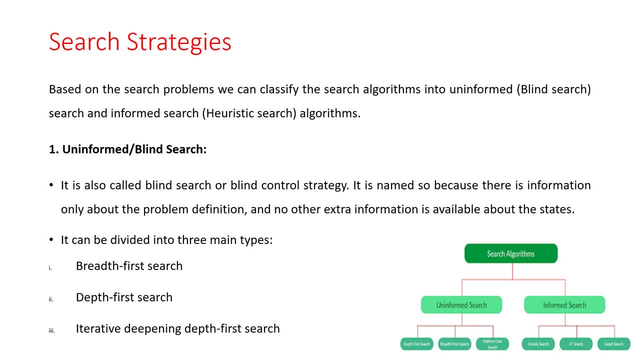 Information only about the problem definition and no other extra information is available about the state. So in this uninformed search does not contain any domain knowledge such as closeness and the location of goal also. okay, So it operates in a brute force way and it is only include the information about how. 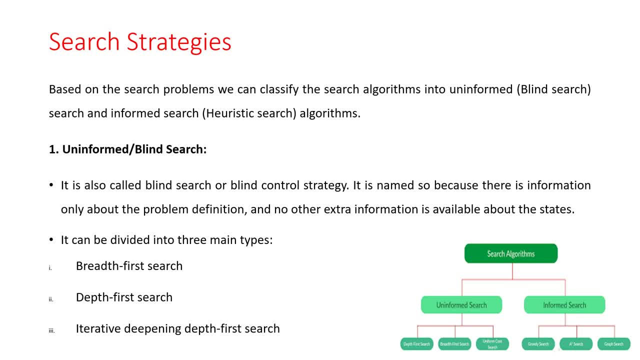 to traverse the tree and how to identify the leaf and goal nodes. So uninformed search applies, a way In which the search tree search without any information about the search space, like initial state operators and the state of the goal, So it is called as a blind search. 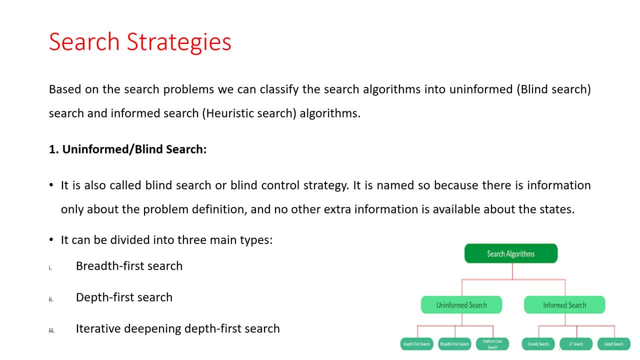 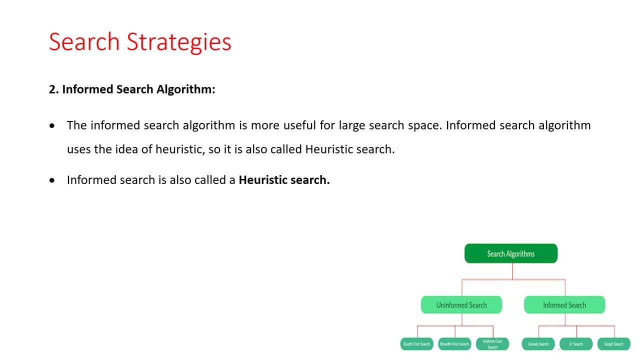 So it is. it can be divided into the three main types, like BFS- breadth first search, DFS depth first search and the iterative deepening depth first search also. And the second type of search strategy is the informed search strategy. So far we have talked about the uninformed search algorithm which look through the search. 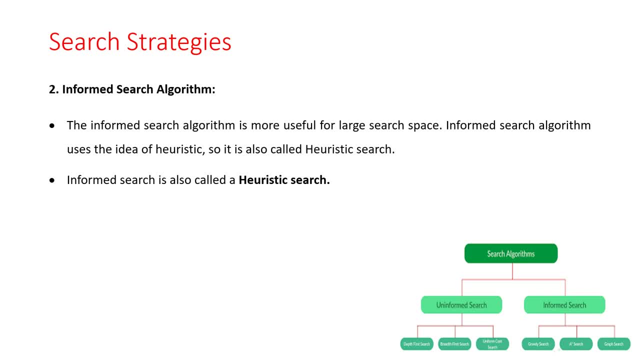 space for all the possible solutions of the problem without having any additional knowledge about the search space. But in the informed search algorithm it contains an array of knowledge, such as how far we are from the goal, path cost and how to reach to the goal nodes, etc. 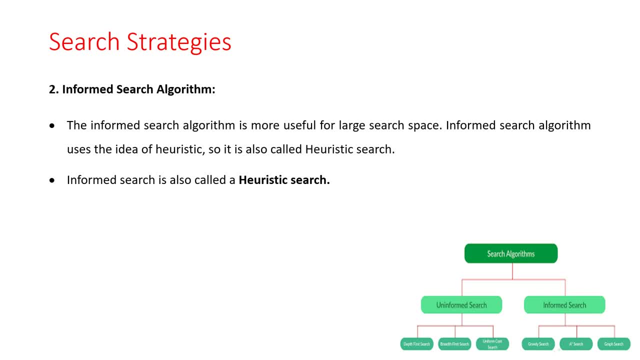 So this knowledge helps to agent to explore. So the informed search algorithm is more useful for the last search space. Informed search algorithm is used for the idea of a heuristic search, So it is called as a heuristic search technique. So informed search, it is also called as a heuristic search. 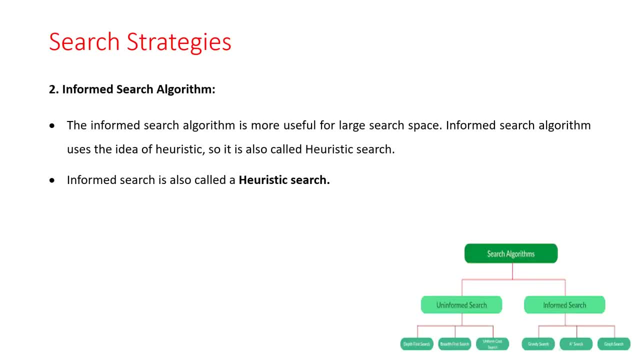 So the heuristic search means what which might not always be guaranteed for the best solution. The heuristic search provide always not provide the guaranteed solution, but guarantee to find a good solution in a reasonable time. They not provide the guarantee for the best solution, but they can provide the good solution. 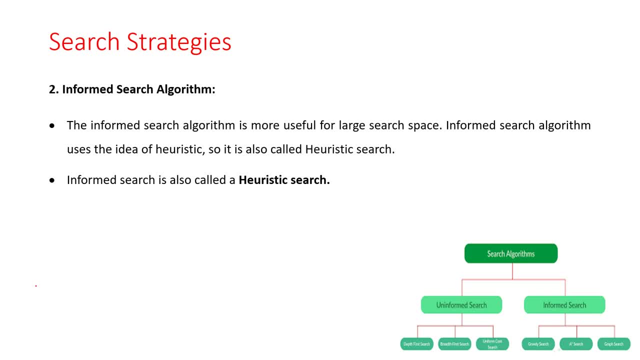 to find the find out the good solution In a reasonable time period. So the BFS, that is, breadth first search, A star algorithm. So these are the different examples for this informed search algorithm. So let us discuss the concept of heuristic search, which is a part of a informed search. 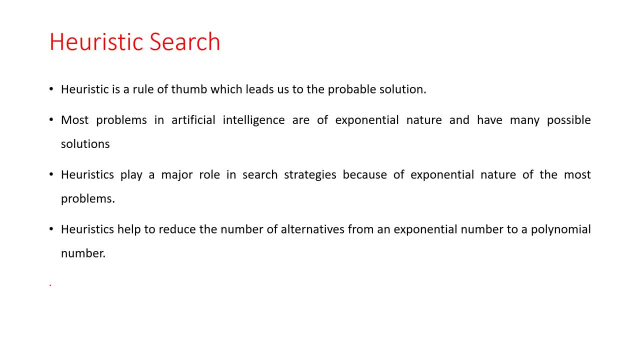 So heuristic is a rule of thumb which lead us to the problem: probable solution. So the most problems in Artificial intelligence are of exponential nature and have many possible solutions. So you do not know exactly which solutions are correct and which solutions are checking. 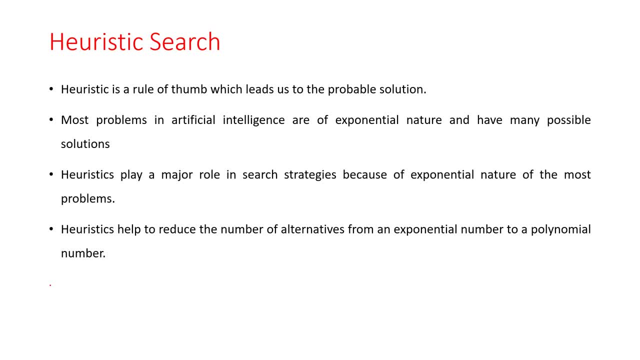 all the solutions would be expensive. So heuristic search is a artificial intelligence search techniques that employs the heuristic for its moves. Okay, We have to search, Do the all the possible rules and then find out the goal state. So heuristics plays a major role in a search strategies because of a exponential nature. 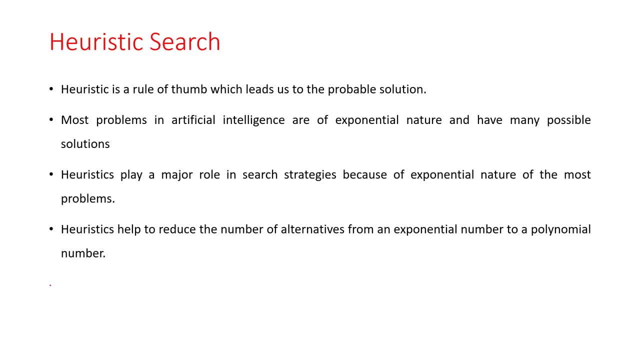 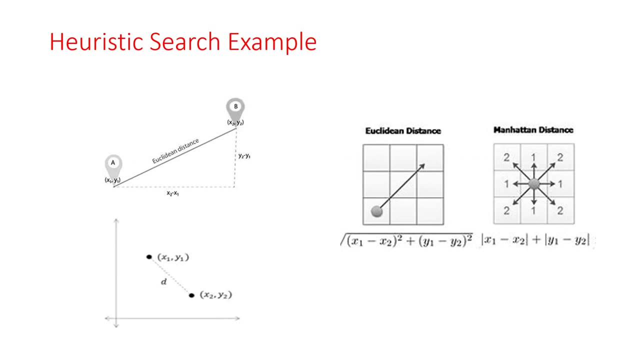 of the most problems. So heuristic help to reduce the number of alternatives from an exponential number to a polynomial number, So see here. So these are the different examples related to the heuristic search. So in an. So in an informed search, the heuristic is a function. okay, heuristic is a function that. 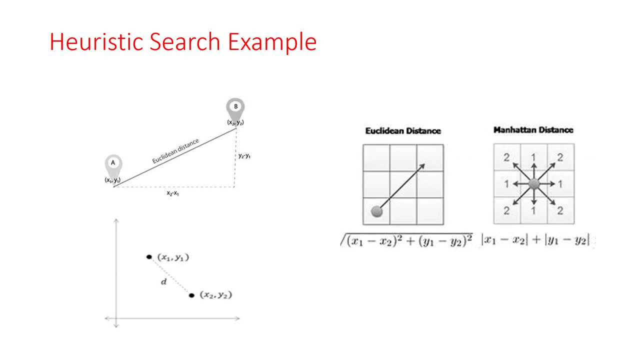 estimate how close to closer state is to the goal state, how a particular state to the goal state. So there are different possible routes. So we have to find out the best possible route to reach to the goal state. For example, there are different distance algorithms like manhattan distance algorithm. 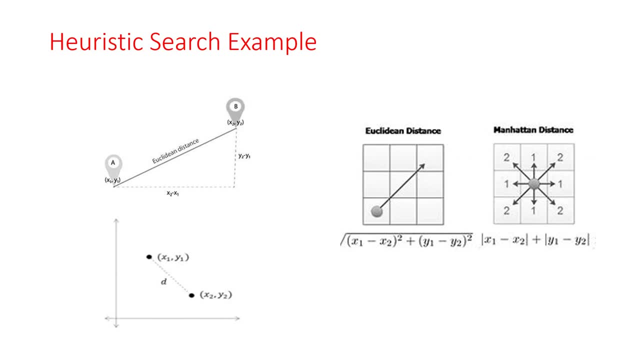 ukrainian distance algorithm. Okay, So by using this algorithm we can find out the distance, minimum distance, from the state to the goal state. So see, here we have to find out the euclidean distance by using this formula: the square root of x: 1 minus x 2 whole square, plus y 1 minus y 2 whole square, and manhattan distance. 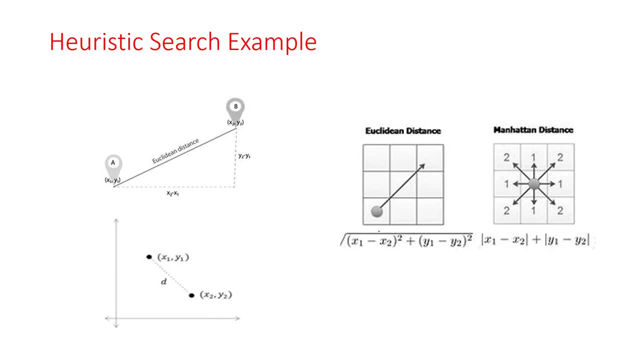 is a mod of x 1 minus x, 2 plus y, 1 minus y 2.. Okay, So, if you are having this type of state, So there is a, one state eight, And another state is a, B and there are another rule state also C, also D also. 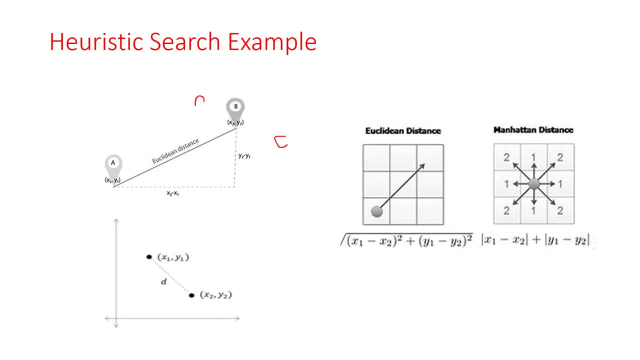 Okay, So we have to find out the distance between a two B also, a two B also, and the a two C also. Okay, So we can find out the euclidean distance here. So by using this formula we can find out the values. 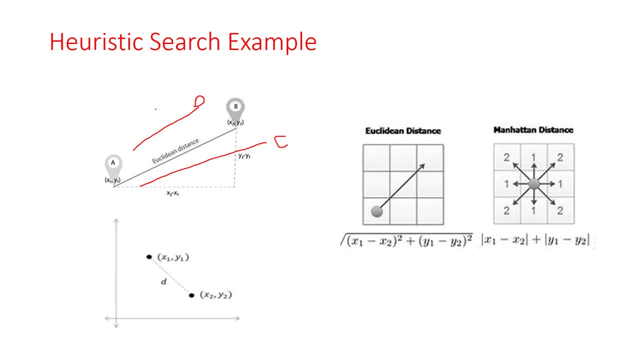 Okay, So here we are getting the value distance is a 7. here we get the distance is a 5 and here we get the distance is a 16.. get the distance is a 8, ok, by using this euclidean distance formula. so so this is a minimum distance. 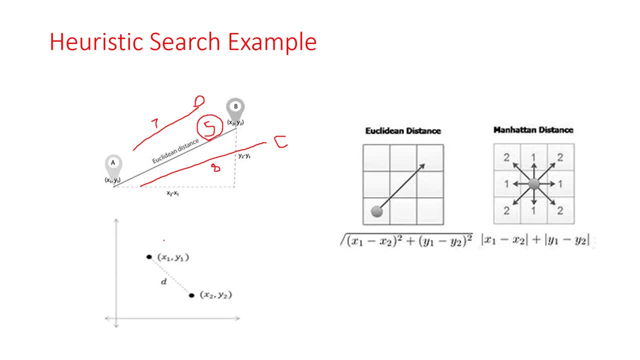 ok, so this is a heuristic search strategy. again, in this example also we can find out a distance between these two points. so there is a point a and there is another point b, so xt minus y2 and x1 and y1 also. so here we are using x1 minus x2, whole square, plus y1 minus y2, whole square. so 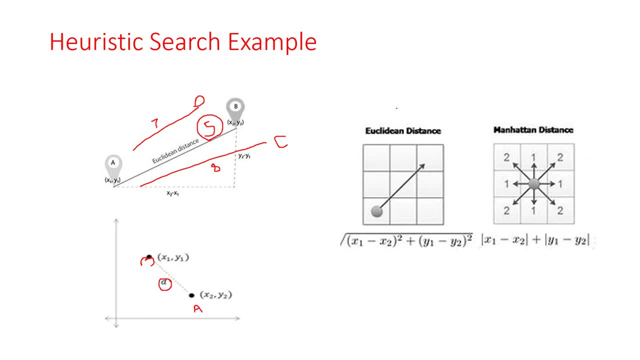 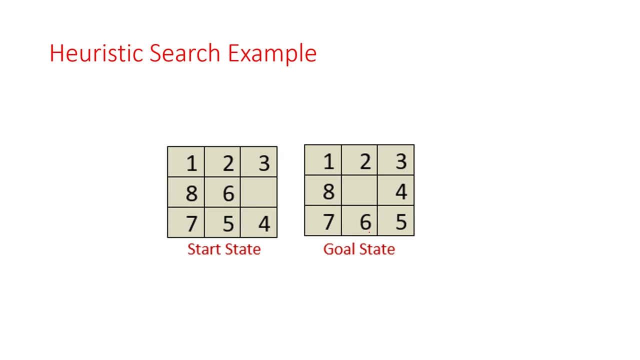 there is a here we get the distance value, ok, by using euclidean distance and we can use the manhattan distance also, ok, so another example is: so there is a star state and there is a goal state, so we have to move these numbers by to reach to this goal state. ok, so he see here from. so there. 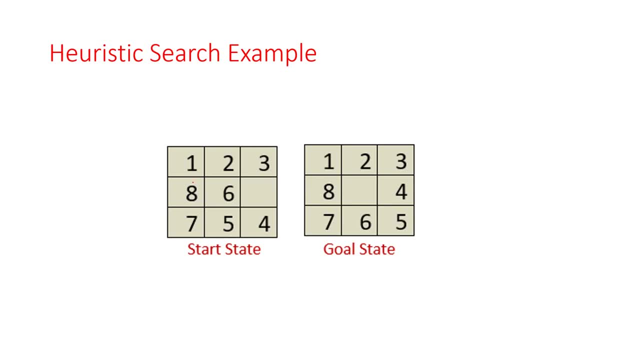 are total: 1, 2, 3, 4, 5, 6, 7, 8, 9. uh sorry, squares, that is. this is our 3 by 3 matrix: 3 rows and 3 columns. ok, and the numbers are 1, 2, 3. 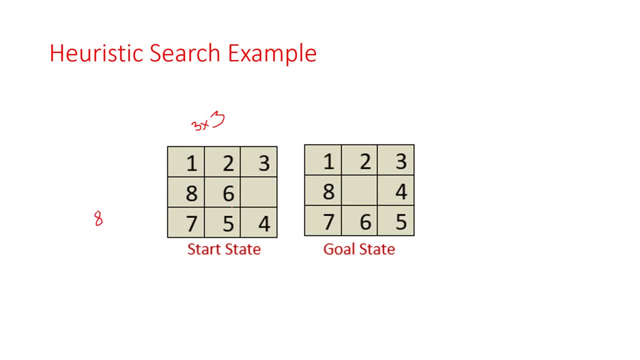 4, 5, 6, 7, 8, so there are total 8 numbers. so we have to move this number uh, where, uh, when we get this type of goal state. ok, so each time we have to find out the path cost, ok, so first path cost is 1. 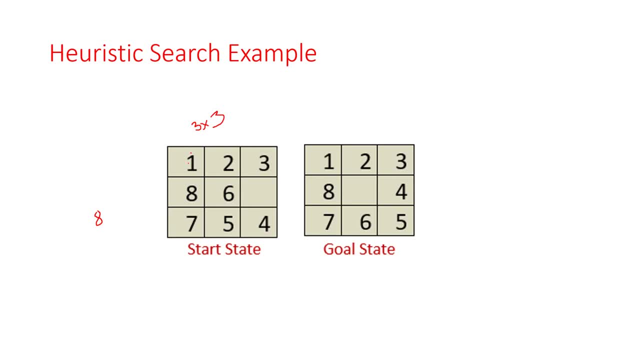 for the one we, so we don't shift this one to upside, downside also, and uh, right side and left side also. ok, so one is as it is, because in the goal state one is, uh in the first position. second is also as it is. third is also as it is. ok. so here the path. cost for is 1: 0 for. 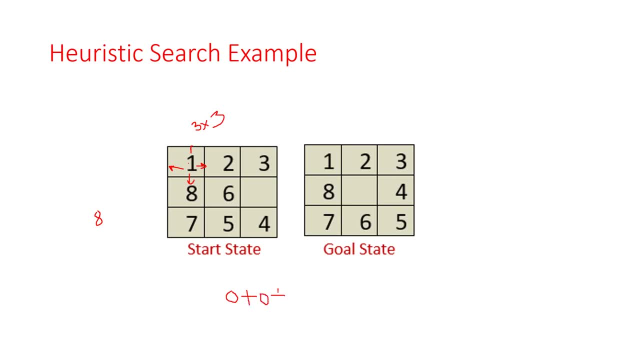 1, path cost is 0 for 2 and path cost is 0 for 3 also, so this is called as a path cost because we have never moved it. so the path cost for 1, 2, 3 is also ok for 2 and for 3 almost. 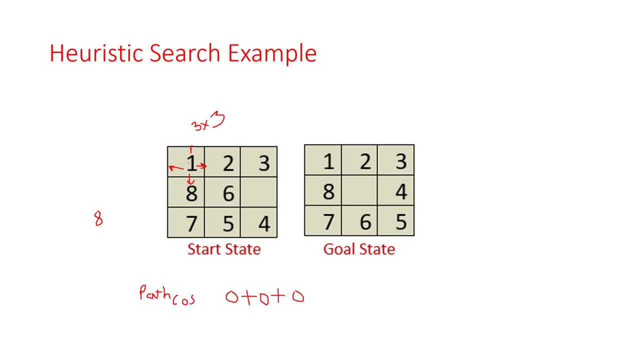 path cost. the path cost for one is 0, 2 is also 0 and three is also zero. ok again, the path cost for 8 is also zero. ok, because we have never moved the path for 8 too. six, six, six, as we have never. 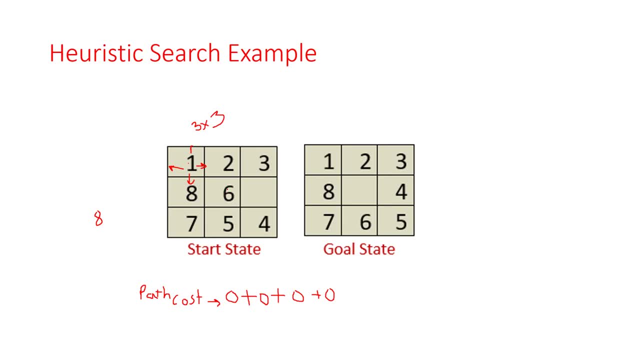 moved it for eight, not yet, because we haven't ever moved it to eight. reached at eight we haven't. So for 6 we have to move because in the goal state the 6 is in the down side. We have to change this 6 to the and then 5 is shifted into this and then 6 is over here. 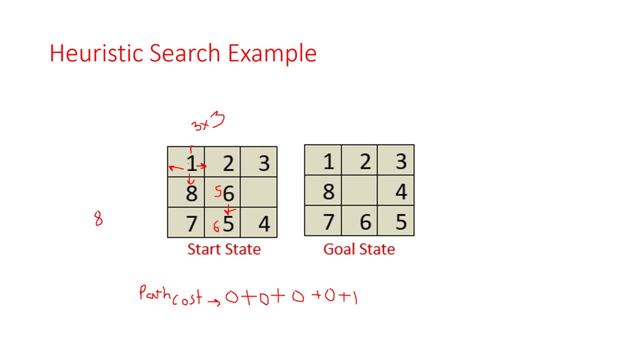 So path cost here will be 1.. After that, 5 is not there. So we have to change this 5 to the shift to the right hand side. Then here we get the blank space and here we get the 5.. But in the goal state 5 is not here. 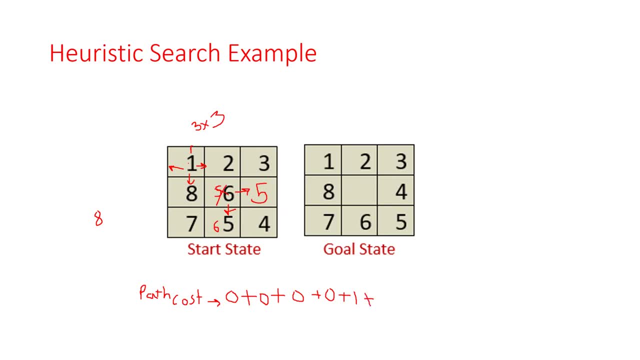 5 is in the down side. So here also we are changing the value of 5, position of 5.. So the path cost is 1.. Again, 5 is not there, 5 is in the down side and 4 is in the middle of this square. 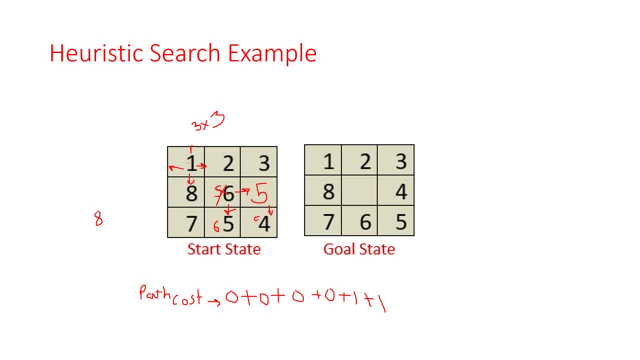 So we have to again shift the 5 in the downwards. 5 is over here and 4 is here. So here we get This type of goal state And the path cost for this changing is 1.. So this is a heuristic search technique. 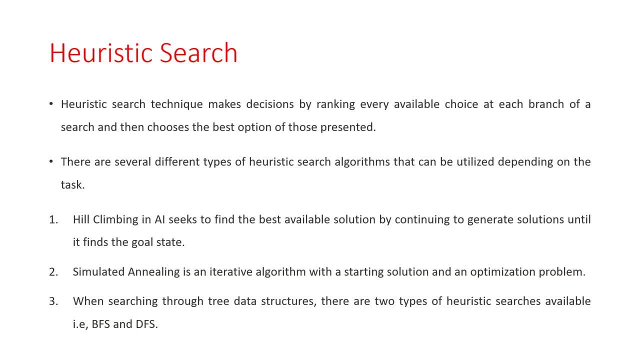 So in the heuristic search technique, it makes the decision by ranking every available choice at each branch of a search and then choose the best option of those presented. So, rather than focusing on finding an optimal solution, like other search methods, If you are using other search method where we get the optimal solutions, 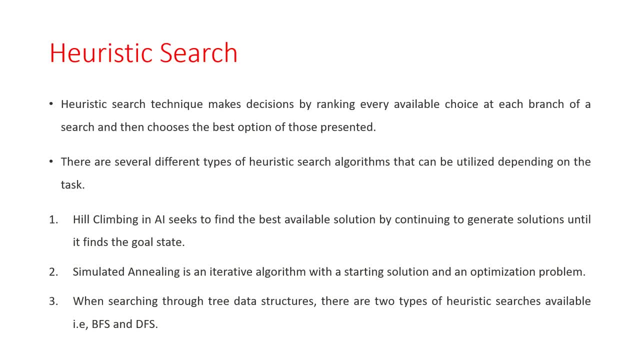 But in the heuristic searching it is designed to be quick, Therefore find the most acceptable option within the reasonable time limit or within the allocated memory space. So there are several different types of heuristic search algorithm that can be utilized, depending on the task. So the type of heuristic search is a hill climb. 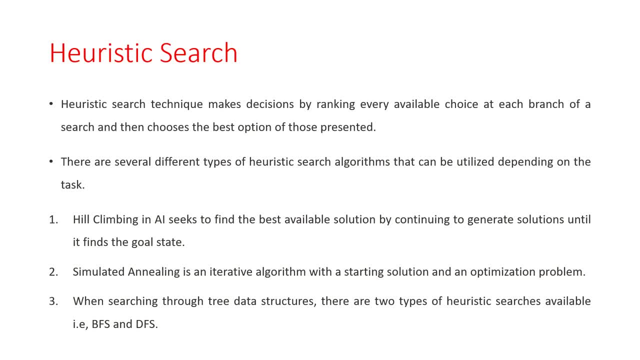 It can be done in simulation, analyzing or BFS or DFS also. So in the hill climbing in artificial intelligence seeks to find the best available solution by continuing to generate the solution until it finds the goal state. So at each step in the process, the algorithm will generate the solution, that it will generate the node and compare the node to the goals. 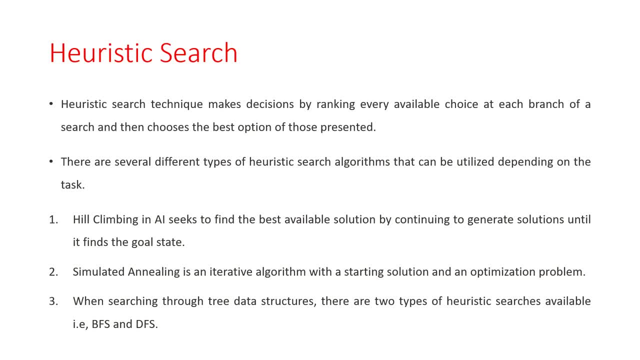 So it is expected. goal state it complete the process. So it is. if it is not so, it will generate the new nodes and repeat until the goal state is found or until it reaches to the local maxima or the state in which all other options are worse than the current one. So this hill climbing search strategies are often utilized. 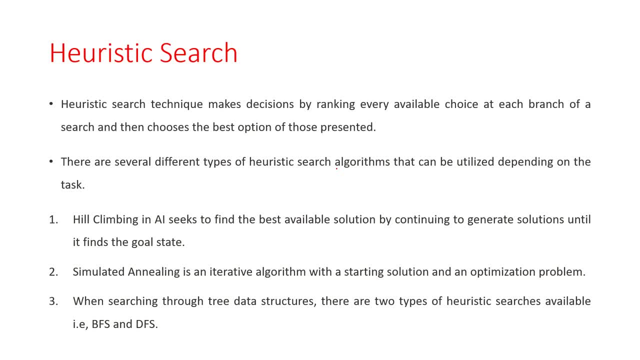 for mathematical optimization, such as traveling assessment problem and which tries to find the shortest possible route between the cell stops. So second type of heuristic search algorithm is simulated analyzing. So it is a iterative algorithm which with the starting solution and an optimization problems. So simulation, analysing it- uses the heuristic function. 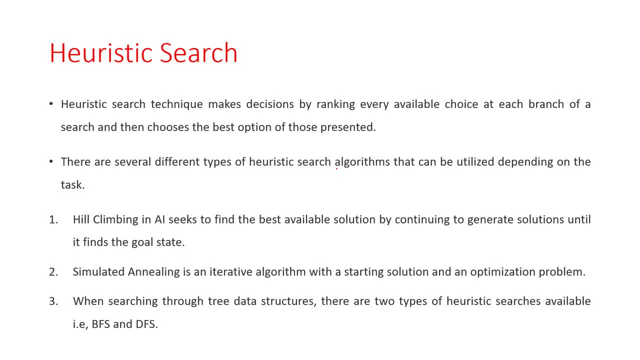 to compare the yea neighboring state of a data and decides between staying in the same stage or moving to the new one. ok, and the third one is the when. the third type of heuristic search algorithm is the BFS and DFS, so when searching through tree data structure. so there are two types. 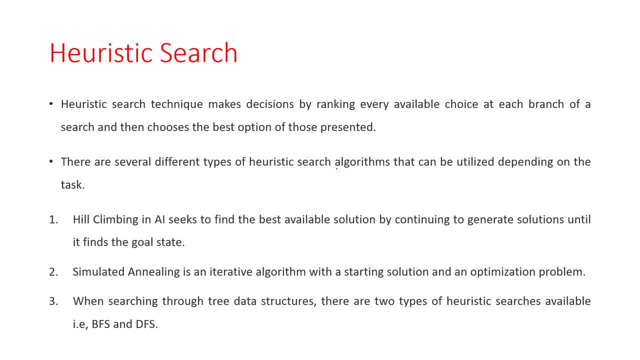 of heuristic search available. that is, the breadth first search and the second one is depth first search. ok, we can. we can search. we can search the. we can search, search any type of heard datas through the BFS and DFS. ok, so then in the breadth first search, we start at determining the root node of the tree and then explore all the. 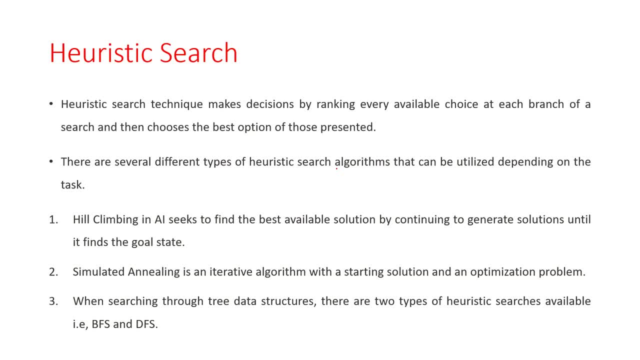 neighbors node at the same depth before moving to the next depth level and in the other hand, in the depth foot would be given a number like First search, it start at the root node and move into the neighboring node. Okay, if you are talking about the breadth, first search, it will start from the root node and then explore the neighboring node, root neighboring nodes from the root node. 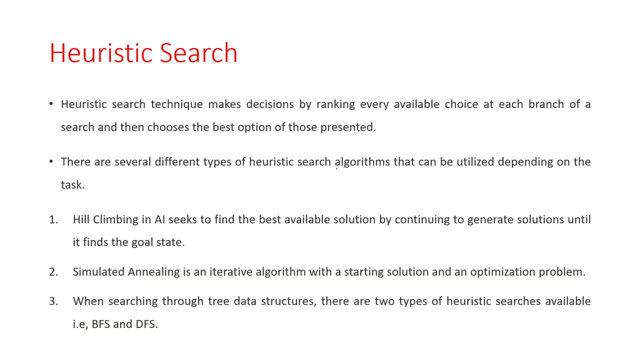 And if you are talking about the depth, first search, if they are starting from the root node and then searching to the depth, wise, until reaches to the final depth before backtracking and moving to the neighboring node. So both these searching types can be used to conduct the topological sorting or finding the connections between the components. 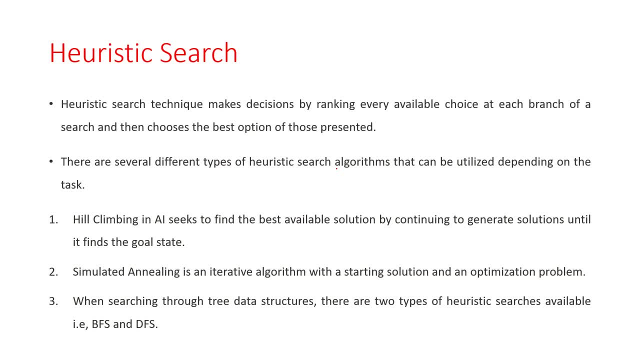 So these are the different types of heuristic search. So this type we can learn in detail in the next lecture. what is mean by hill climbing, how this hill climbing works. what is mean by simulated annealing, how this simulated annealing is work, and BFS and DFS also. 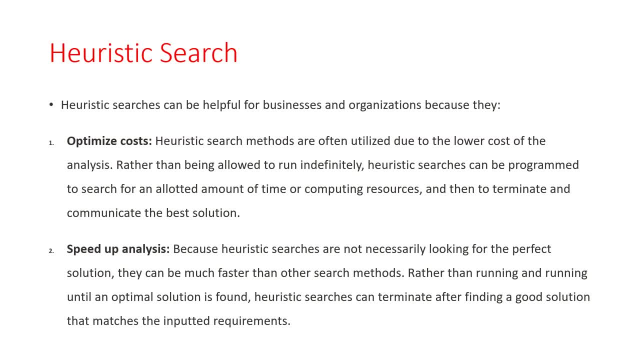 So heuristic searches can be helpful for business and organization because they have optimized cost and they have the speed of analysis. So in the optimized cost, the heuristic search methods are: 1. Often utilized due to the lower cost of the analysis rather than being allowed to run identifiably. and the heuristic searches can be programmed to search for an allotted amount of time or computing the resources and then to determine and communicate the best solution. 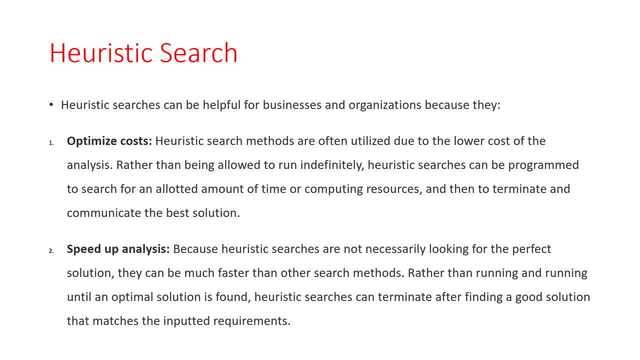 So this is the optimization cost. Another thing in the heuristic search, that is the speed of analysis. So because the heuristic searches are not necessarily looking for the perfect solutions, they can be much faster than other search methods. So rather than running and running until the optimal solution is found, the heuristic searches can terminate after finding the good solution that matches the inputted requirements. 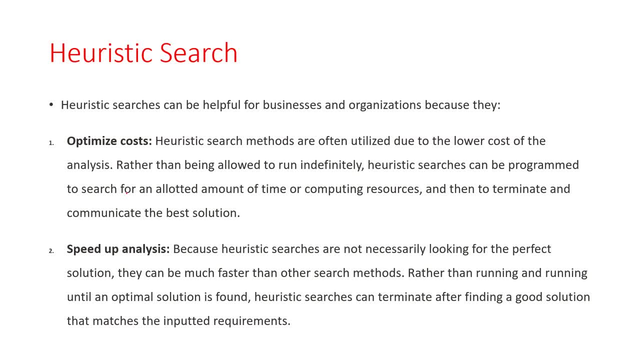 So these are the two heuristic searches helpful for the heuristic search. Now let's talk about the heuristic search. Heuristic search is basically the way how the heuristic search takes you to the right place in your business and organization. that is, optimized cost and the speed of analysis. 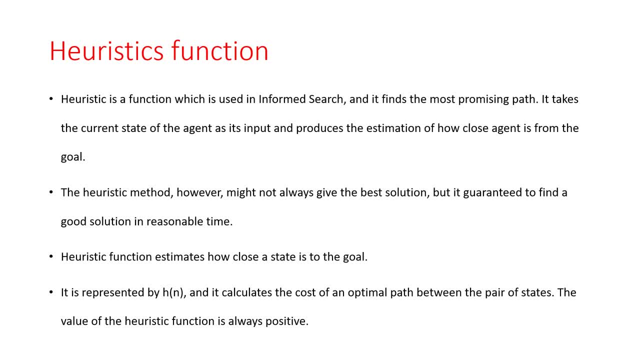 So next thing is: what do you mean by heuristic function? Okay, if you're solving the heuristic search technique, So in that case we use some heuristic function. So heuristic is a function which is used in the informed search and it finds the most promising path. 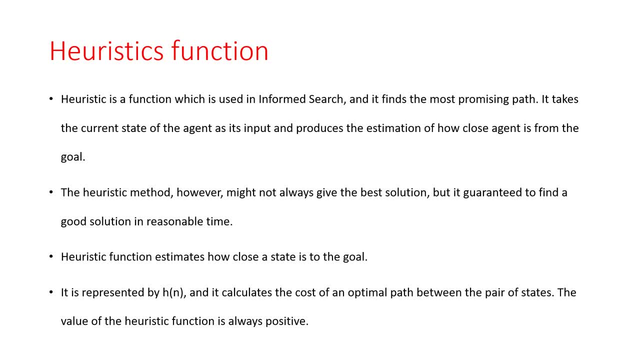 So it takes the current state of the agent And it's input And produces the estimation of The business And the organization And the optimization. So the following is another thing which is used to calculate the heuristic search method To find the most promising path. 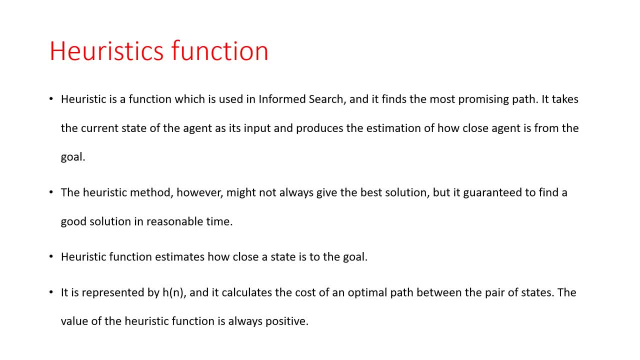 So what is heuristic search method? how the close agent is from the goal. So this heuristic method, however, might not always give the best solution, but it guarantees to find the good solution in a reasonable time period. Okay, so heuristic function estimates how close a state to the goal state. So it is. 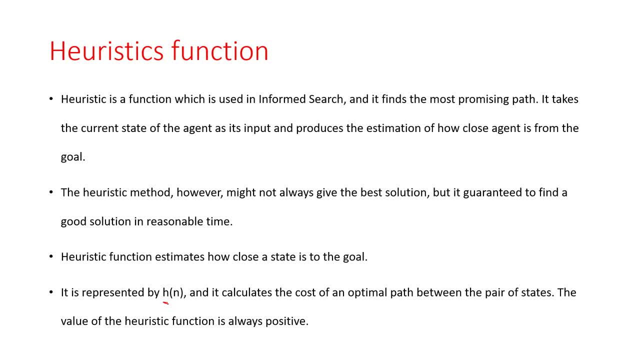 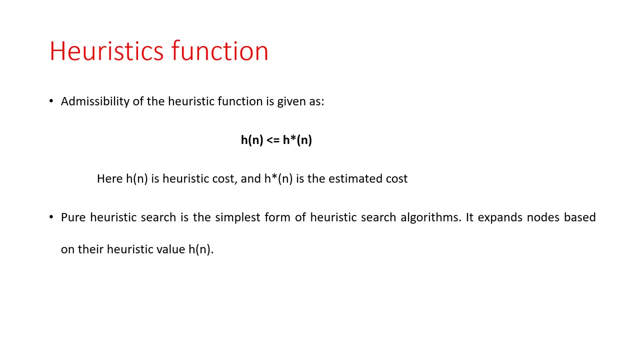 represented by h of n. So h of n is the heuristic function, and it calculates the cost of an optimal path between the pair of states. The value of the heuristic function is always positive. So here, so I also, administrability of the heuristic function is given as h of n is less. 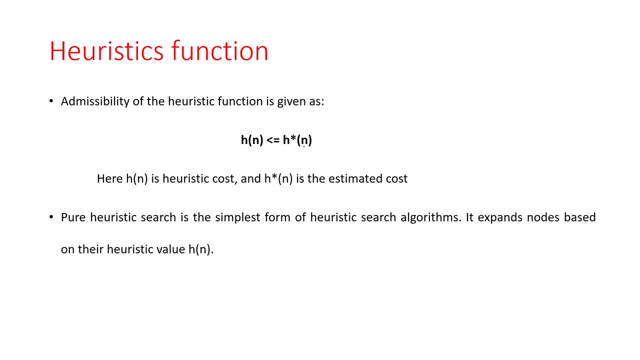 than equal to h into n. Here the h of n is the heuristic cost and h into n is the estimation cost. Okay, so pure heuristic search is the simplest form of a heuristic function. So pure heuristic search algorithm. it expands node based on the heuristic value. Okay, so